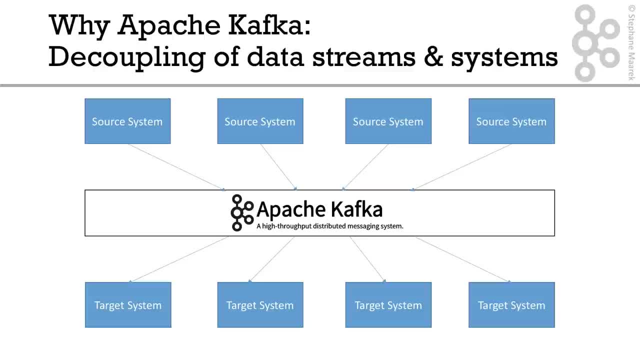 comes in. So Apache Kafka allows you to decouple your data streams and your systems. So now your source systems will have their data end up in Apache Kafka, while your target systems will source their data straight from Apache Kafka, And so this decouples your data streams and your. 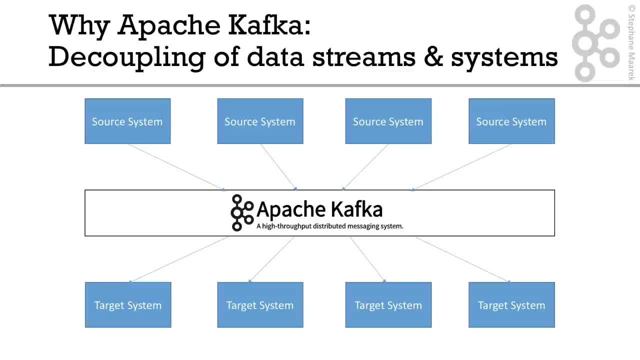 systems. So decoupling is what is so good about Apache, Kafka and what it enables is really really nice. So, for example, what do we have in Kafka? Well, you can have any data stream you can think about. For example, it could be website, events, pricing data, financial transaction user. 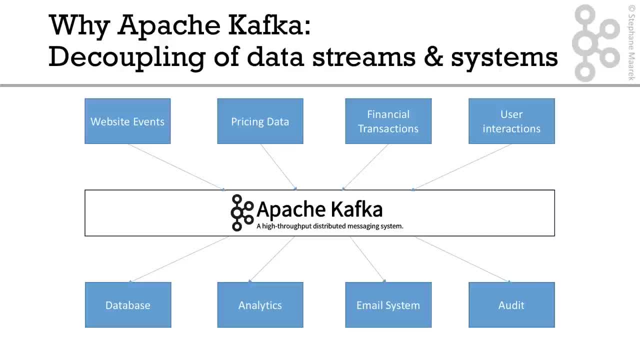 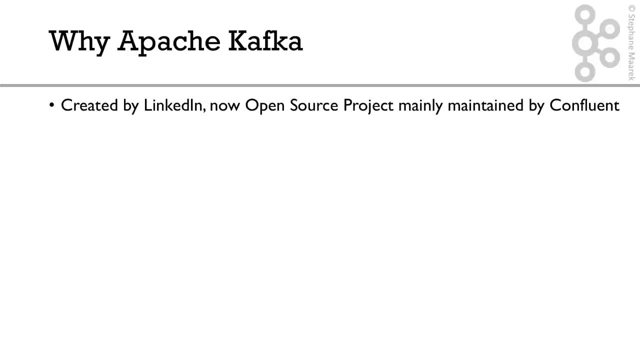 interactions and many more. Additionally, once the data is in Kafka, you may want to put it into any system you like, such as a database, your analytics systems, your email system or your audit. So why would we even use Apache Kafka, right? Well, it was created by LinkedIn and it's now an 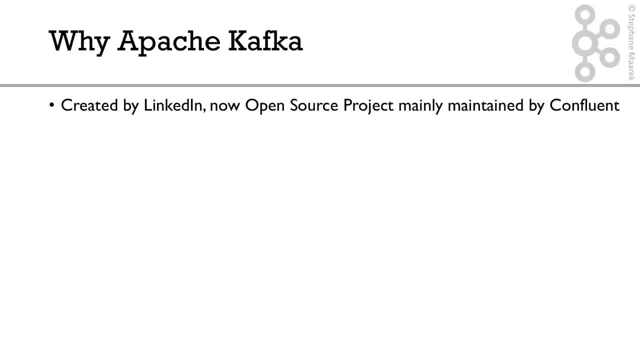 open source project mainly maintained by a private company called Confluent, but it's under the Apache stewardship. It's distributed, resilient architecture and fault tolerant and basically it scales. It scales horizontally- There are Kafka clusters with over 100 brokers. It can also scale. 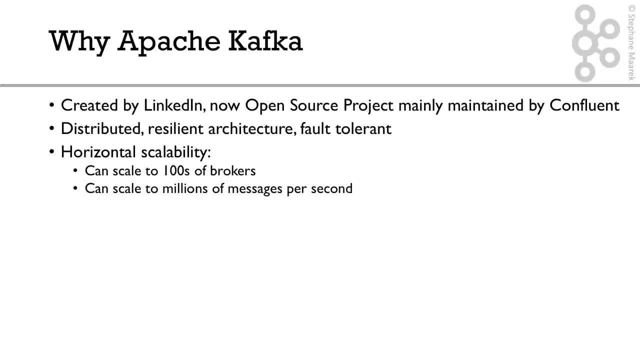 and it's proven by LinkedIn and many other companies that it can scale to millions of messages. So what do we have in Kafka? Well, the first thing we have in Kafka is the latency. So if you want to use Kafka, you can use the latency to exchange per second. That's quite a lot of scale. It is extremely. 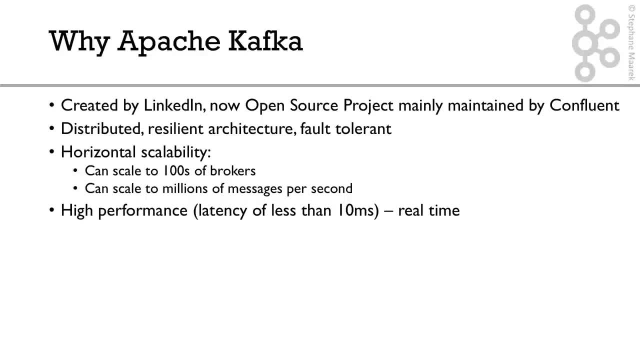 high performance. The latency to exchange data from one system to another is usually less than 10 milliseconds if you have good machines, And this is what we call real time. Real time means that the latency is really, really low Overall. don't believe me right, You can believe 2,000 plus. 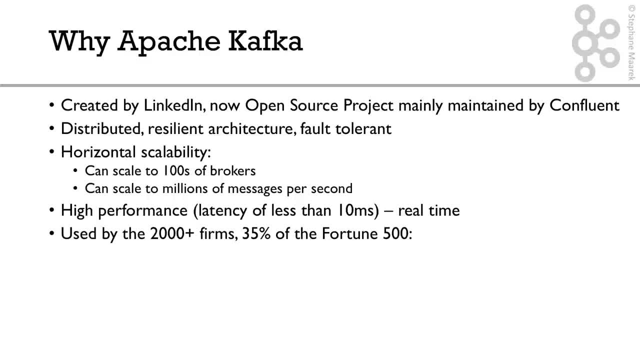 firms- 35% of the Fortune 500- that use Kafka, such as LinkedIn, Airbnb, Netflix, Uber, Walmart and so many others. right, So you can use Kafka to exchange data from one system to another, And this is not just in the box for you guys to use Kafka. You can use Kafka to exchange data for your business. 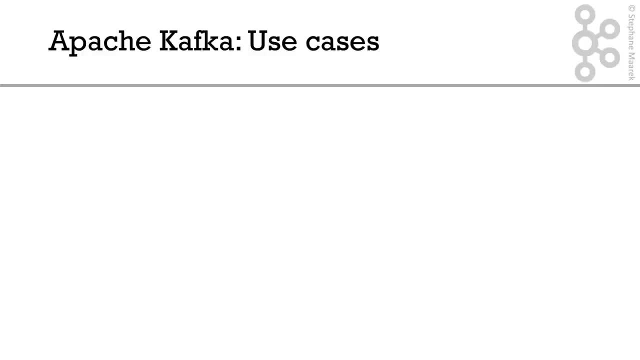 right, Everyone uses Kafka or is thinking about using Kafka, and you should learn Kafka and you are at the right place. So use cases for Apache Kafka. Well, it could be a messaging system. It could be used for activity tracking or to gather metrics from many different locations, such as your examples. 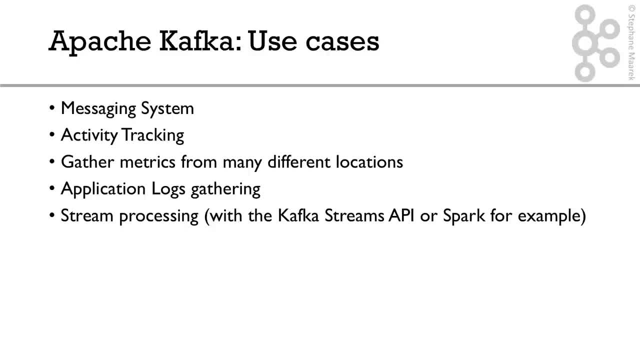 or your IOT devices, gather logs from your applications stream processing and we'll see that we can use the Kafka Streams API for that bases and your systems by decoupling them or perform big data integrations, for example, with Spark, Flink, Storm, Hadoop and other big data technologies. So this is quite a wide array of 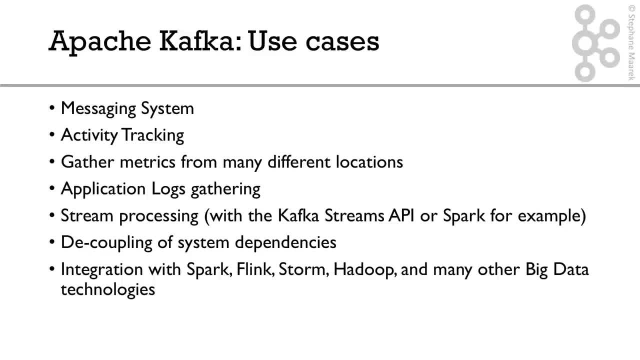 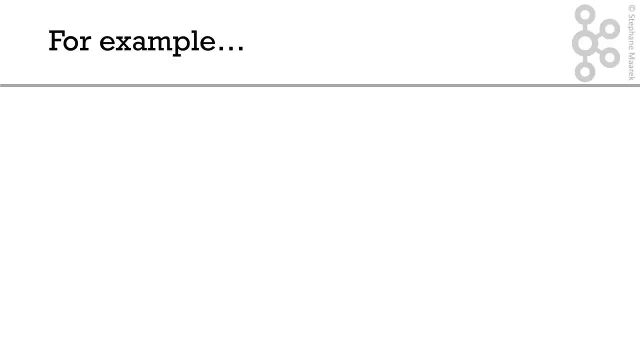 use cases and this is why so many companies are using Apache Kafka as their backbone in their company. Now, if I want to give you a concrete example that get you a bit excited about Kafka, that make you understand what Kafka is used for, Netflix is using Kafka to apply recommendations. 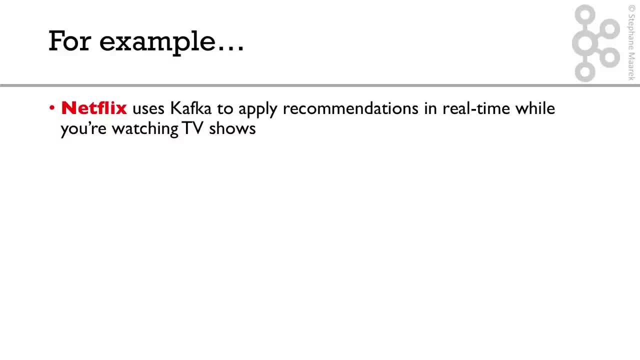 in real time while you're watching TV shows, and this is why, basically, when you leave a TV show, you'll get a new recommendation right away. Uber uses Kafka to gather user taxi and trip data in real time to compute and forecast demand and compute the almighty search pricing in real time. 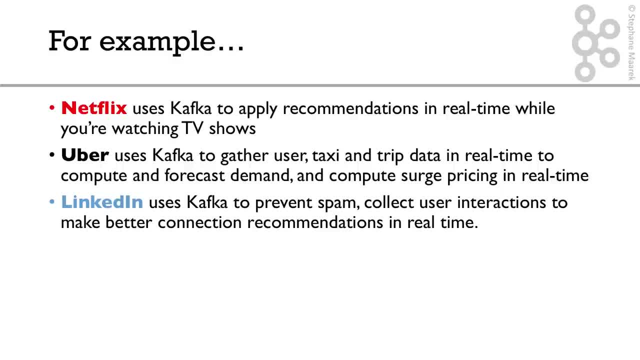 So Uber uses Kafka extensively, LinkedIn uses Kafka to prevent spam and their platform collect user interactions and make better connection recommendations. all of that in real time, Basically, as you can use that. as you can see, all these companies are using Kafka so that they can make real-time recommendation, real-time decisions, give you real-time insights to their 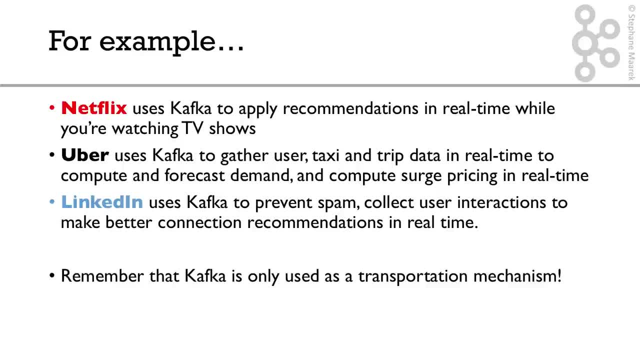 users, and this is why it's so good. Now remember that in this, Kafka is only used as a transportation mechanism. People need to still write their applications or web applications to make things work, but Kafka is really good at making real-time decisions. So if you want to make real-time, 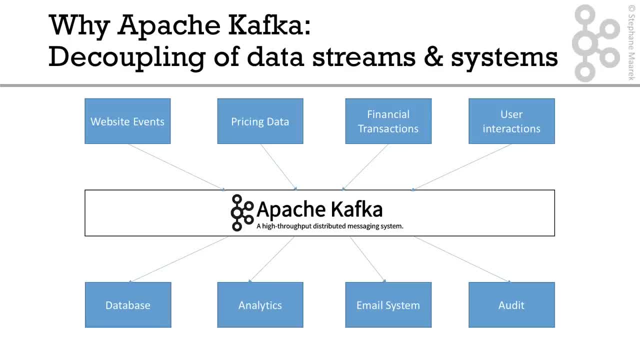 decisions and making your data move really fast at scale in your company. So that's it for a quick introduction to give you some insights about what Kafka is, how it works and where it sits in companies and how they use them. So in the next lectures and an entire course you're going to 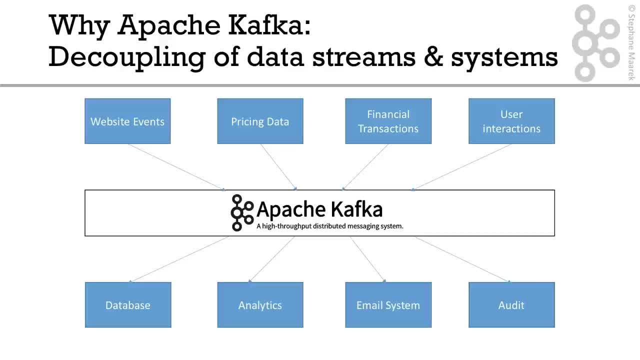 accumulate so much knowledge and practice around Kafka. but I hope that in these first five minutes you really understand what we're going to talk about for the rest of this course- and I hope you're excited- I will see you in the next lecture.